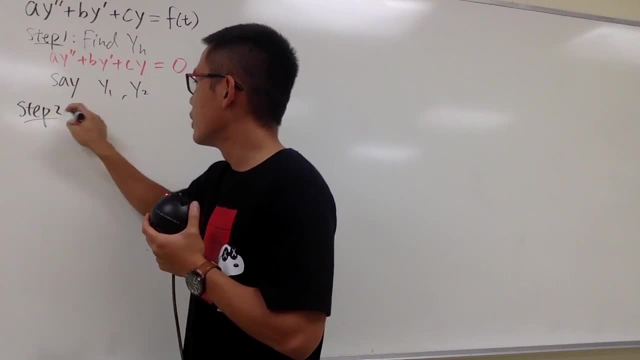 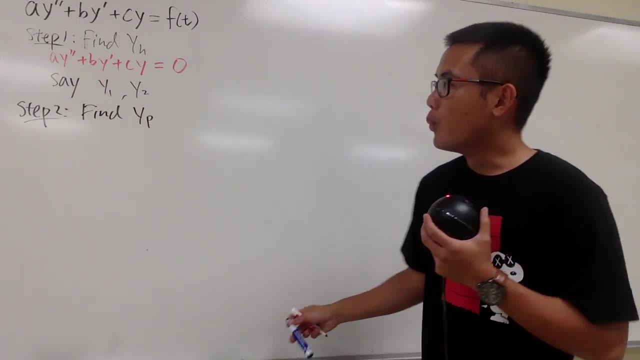 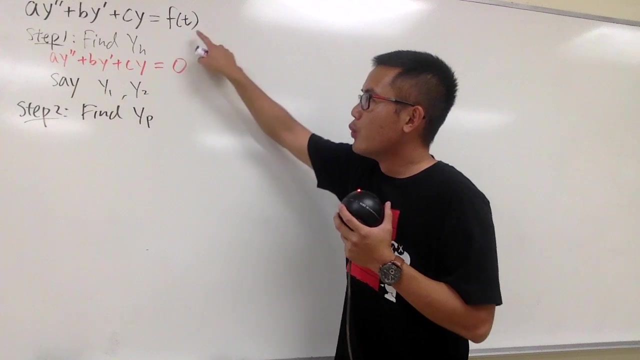 And now step two: We have to find the particular solution. so that's yp. And now let's think about it. We have two solutions already right: y1, y2.. We have to find a new one, And, by the way, we could have done this with an undetermined coefficient. 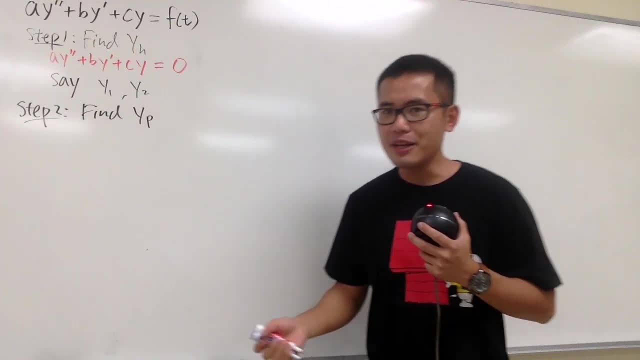 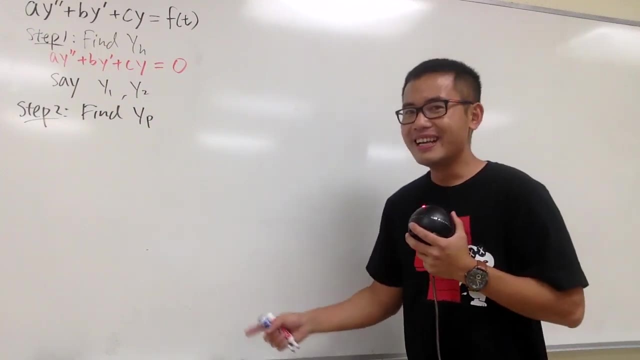 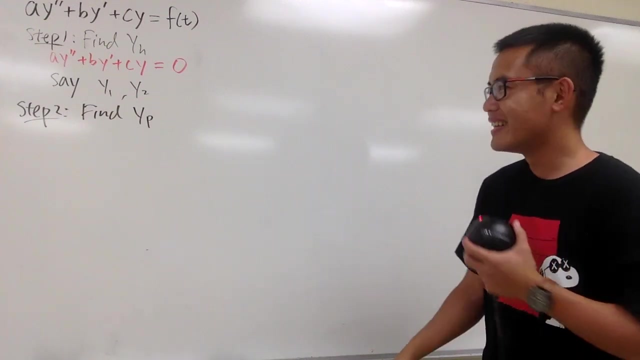 If f of t is sin, cosine or maybe exponential or maybe polynomial, right? If you're willing to use the following method, in fact, you can deal with f of t being tangent and also maybe secant or whatsoever, right? So it's really cool, right here? 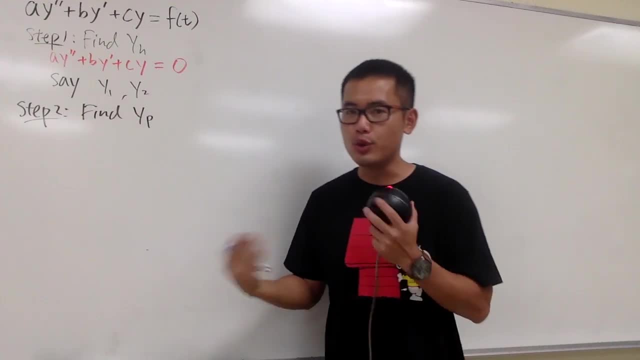 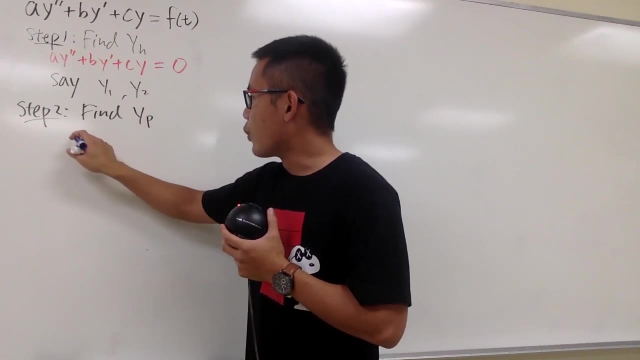 Anyway, we know two solutions already. How can we find a new one? This sounds like the method of reduction, isn't it? If I know y1 already, just think back to the method of reduction Of water. Reduction of water, okay. 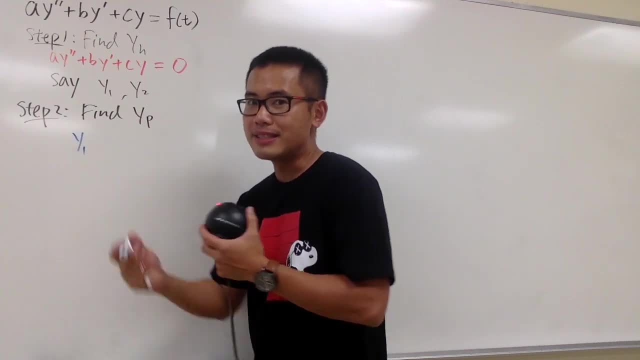 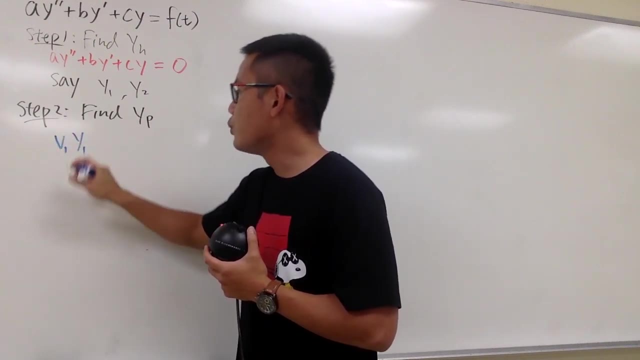 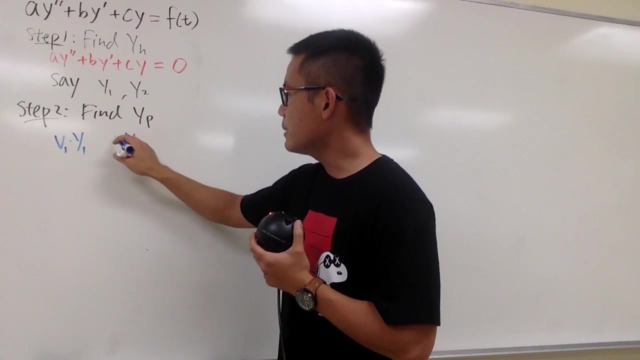 You look at y1, and you multiply that by a function and that's how you are going to produce the new function for the solution, right? So y1 will multiply to say v1,, all right. But I also know y2 is a solution as well, so I'll put down y2, and let's multiply this by v2.. 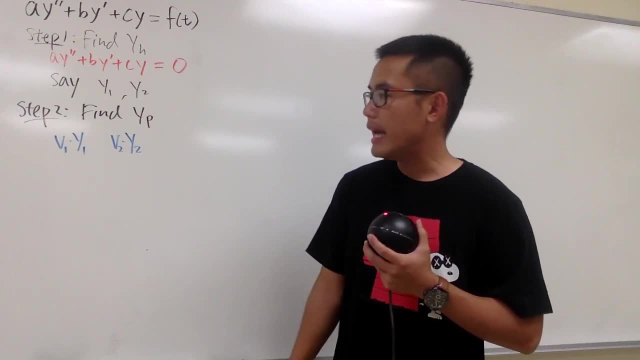 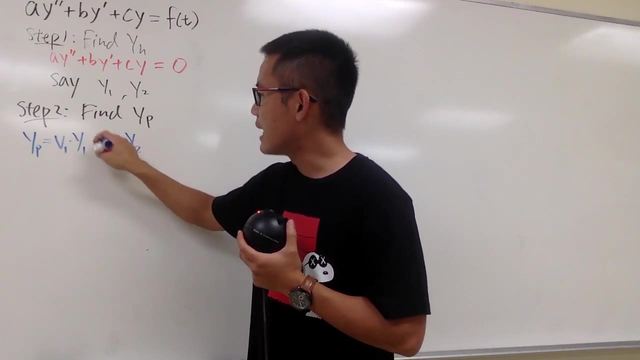 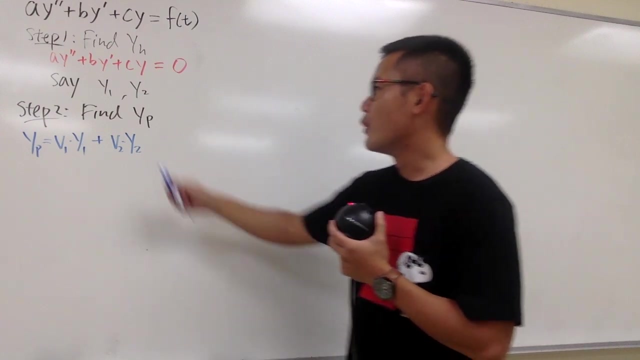 v1, v2,. they are both functions of t and, in fact, for yp. in this case this is equal to v1, y1, plus v2, y2. And this is very similar to the idea of reduction of waters, but this time we know two solutions already to find a 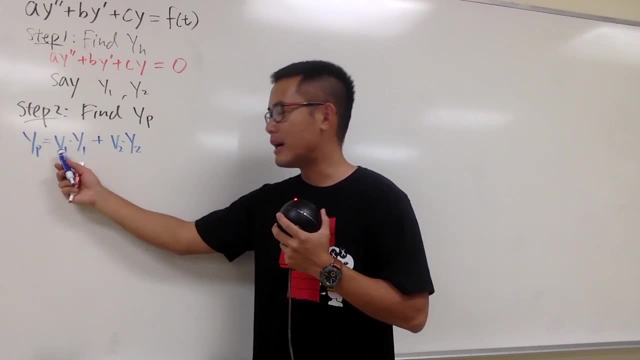 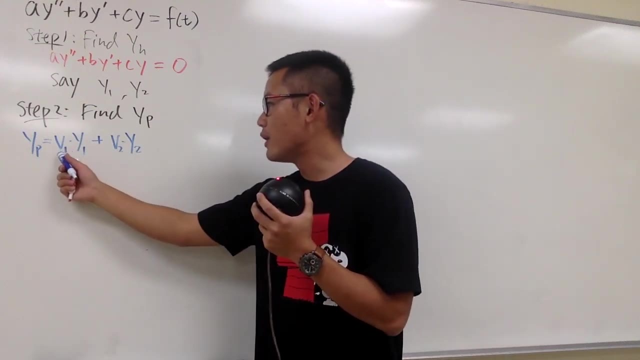 new one, yp. in this case You multiply the first one by another function, v1,, and then you multiply by y2, it's v2.. And our goal is to find out what v1, v2 are. y1, y2 will be really easy. 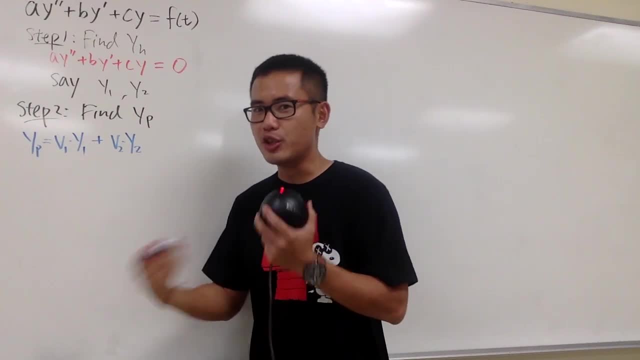 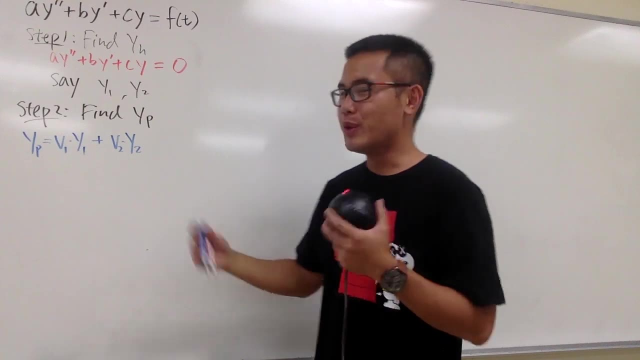 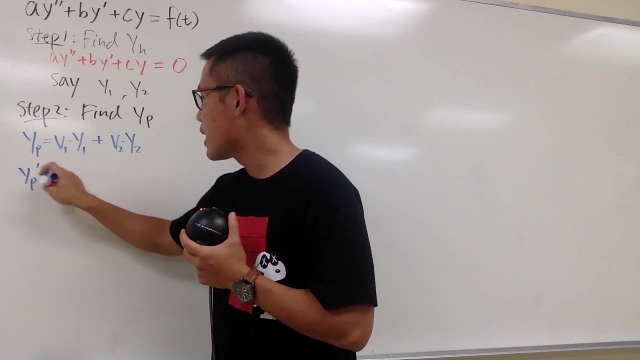 Anyway, we have this. This is just a general form. We just have to differentiate this twice, Plug in and then see what we can get from there. right Anyway, product rule, product rule. let's get to work First. derivative, right here, yp', this is going to be. 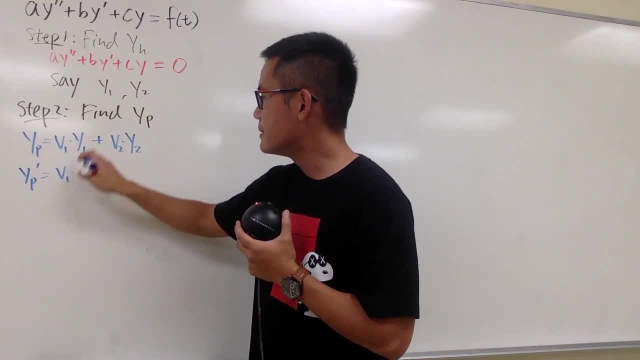 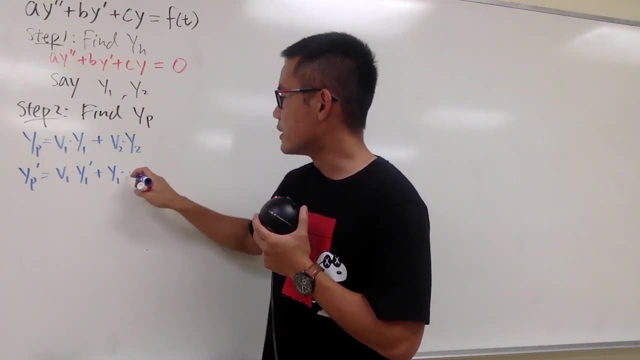 I will keep the first function, which is v1, times the derivative of the second, which is y1'. plus, I will keep the second function, which is y1, times the derivative of the first, which is v1'. All right. 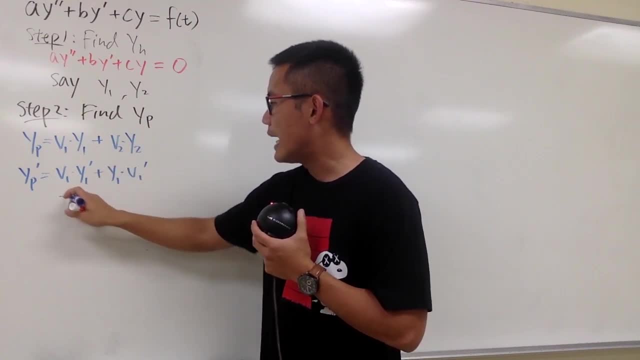 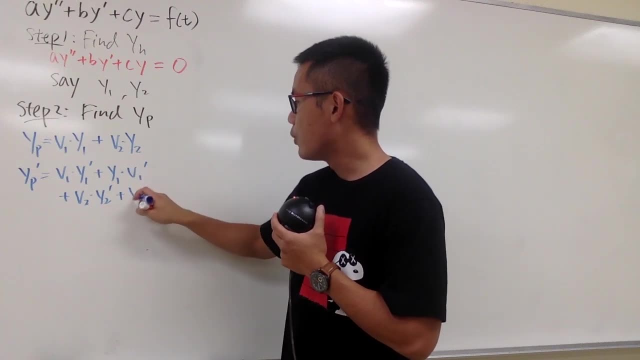 And next up this. So I'm going to put it down here. I will add: I'll keep v2, and I'll multiply by the derivative of the second, which is y2' and then, plus, I'll keep y2,. 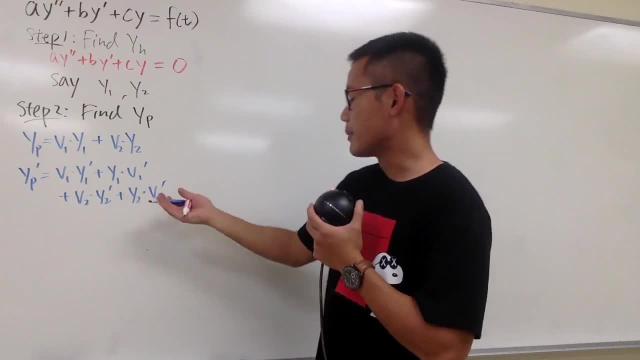 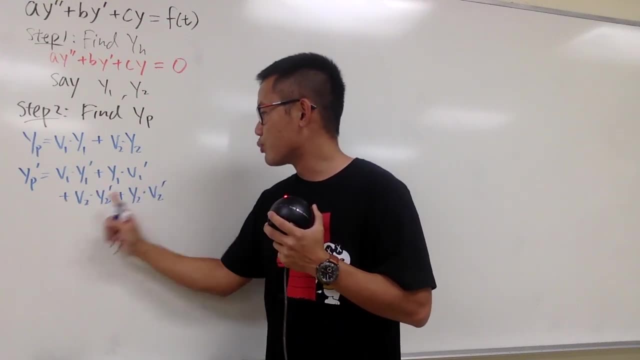 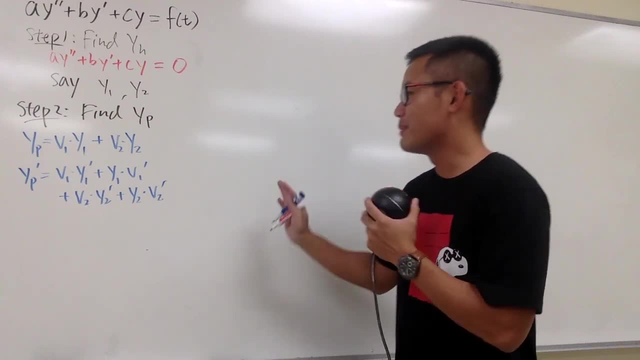 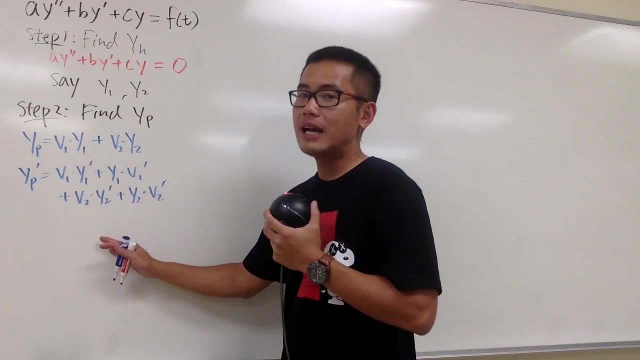 But let me tell you: no, no, no, no. Let's think about this before we continue. Okay, so here is the deal. If I just want to differentiate this, I will end up with a lot of things, right, A total of eight things. 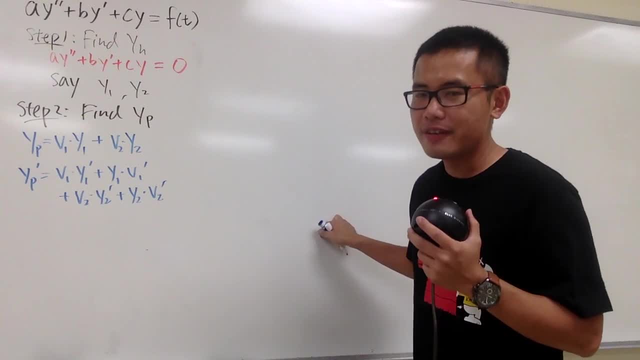 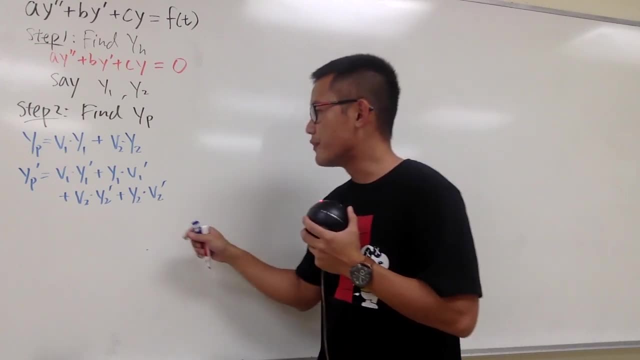 I don't want to go through that, and this is a condition that we're going to impose right now. What I want to do is I want to avoid the second derivative of v's. Right here, I see v1'. right here, I see v2'. 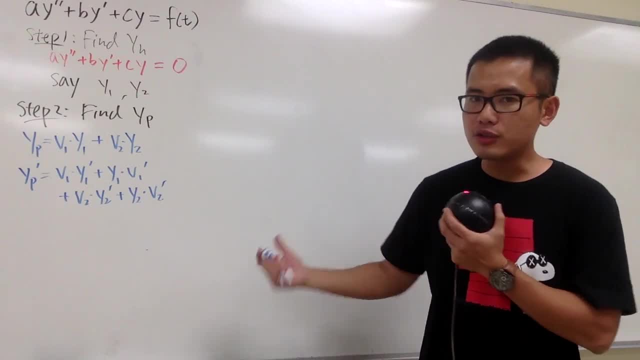 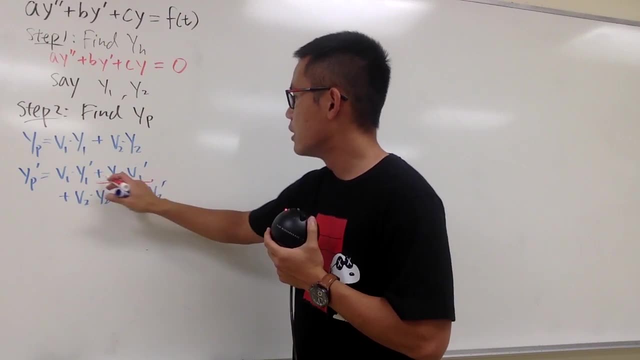 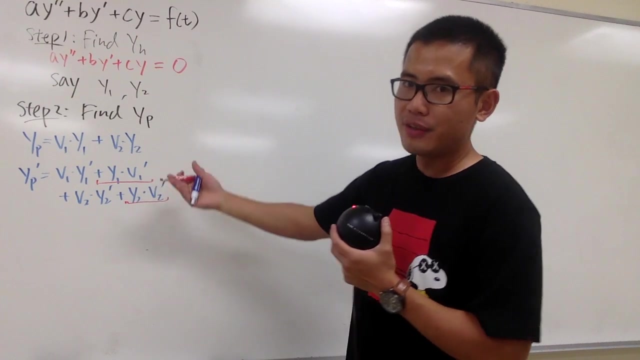 I want to avoid the second derivative of the v functions, So this is the condition I'm going to impose. I see this is what we have right here: y1', v1', y2', v2', right, They both have the v derivatives, right. 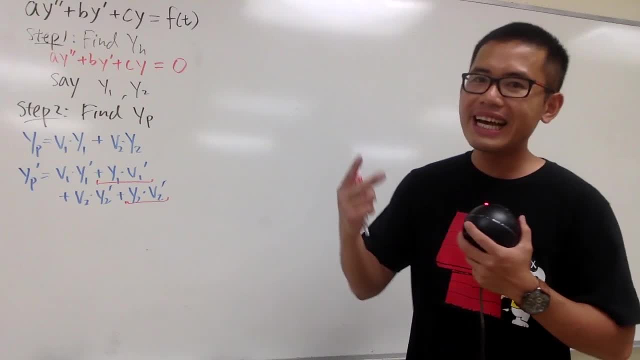 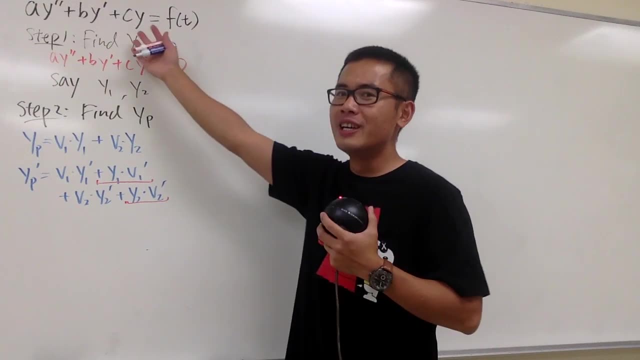 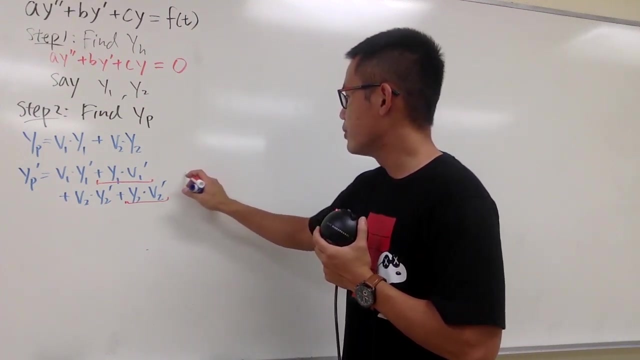 Imagine, if you look at this and differentiate this again, you end out with a second derivative for the v's And you end out with like a second-order differential equation instead of a second-order differential equation. let's not do that. so this is the idea, this is the condition I'm going to. 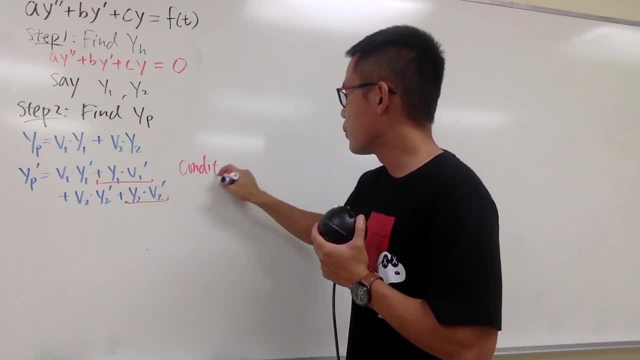 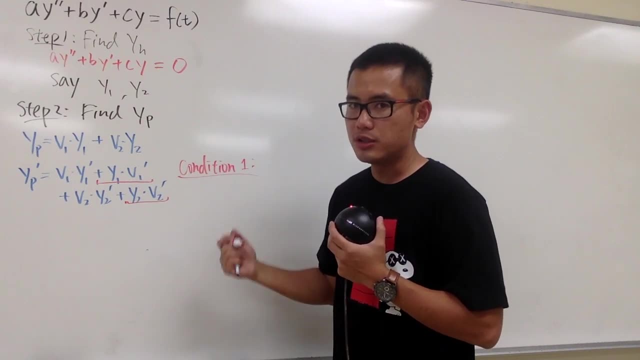 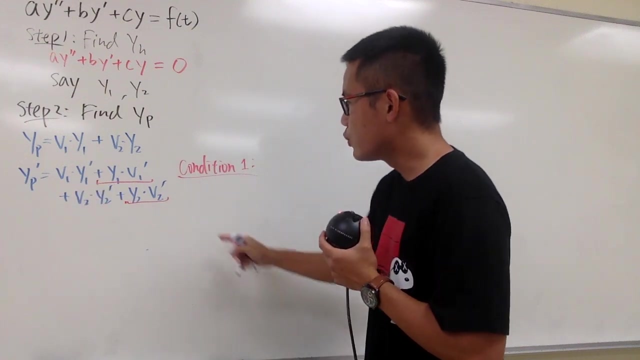 impose. here is condition number one. all right, so I want to assume that this and that add up to be zero, so I can just ignore that and YP will be just this and that YP prime will be just this and that. okay, so condition one, let me write it. 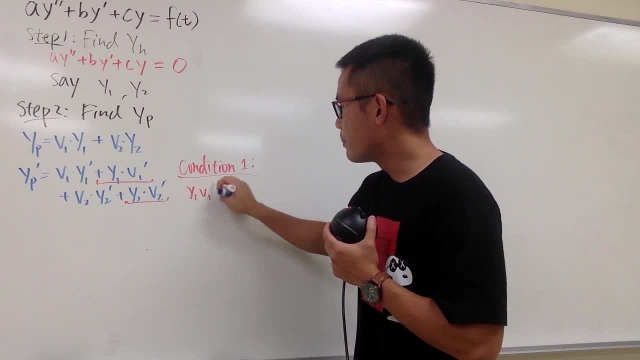 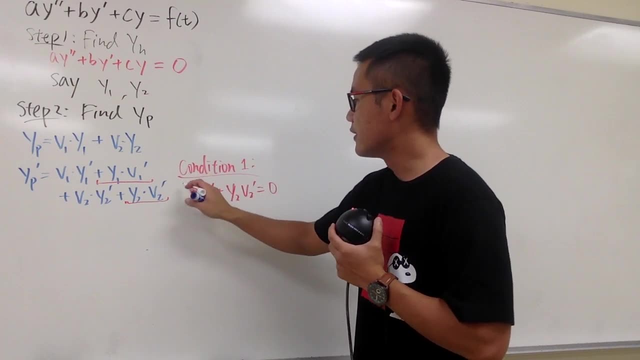 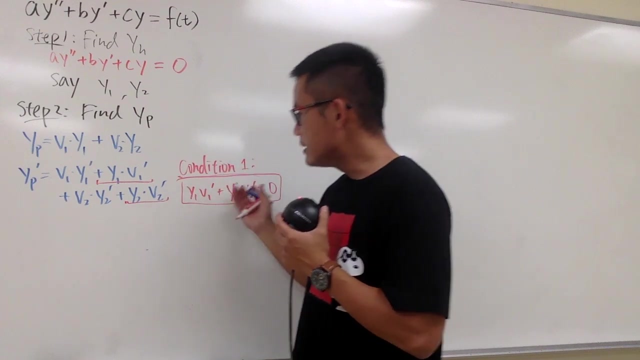 down. I want to have Y1 B1 prime plus Y2, Y2 B2 prime. this equals to zero. this is the first condition that I want to have. okay, so let me box this right here. and because this is equal to zero, now right, so I can rewrite this for you guys: YP. 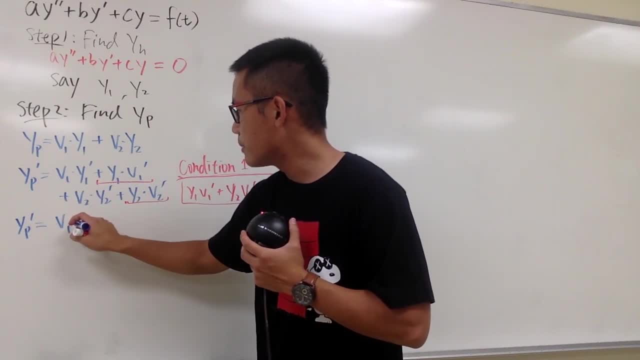 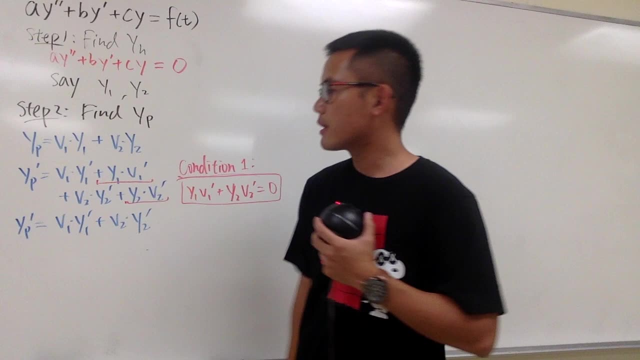 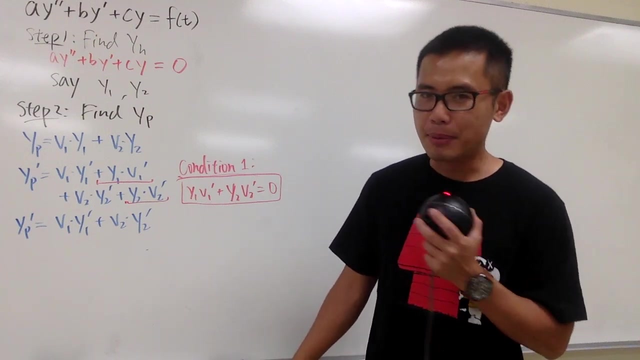 prime is just equal to B1 times Y1 prime plus B2 times B2 times Y2 prime. that's YP prime. and now I can look at this and differentiate this again. I can get YP double prime right. so let's get to work. this is slightly. 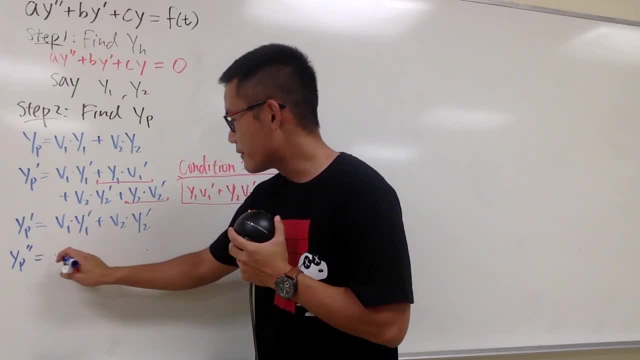 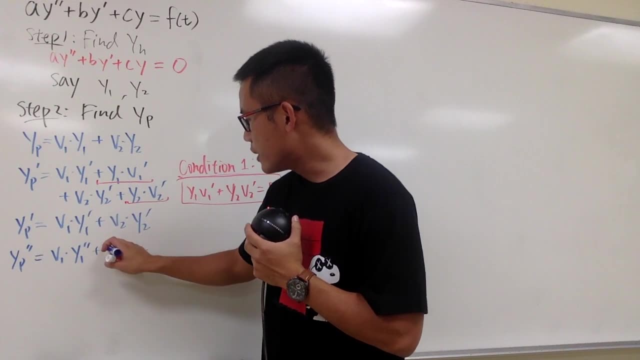 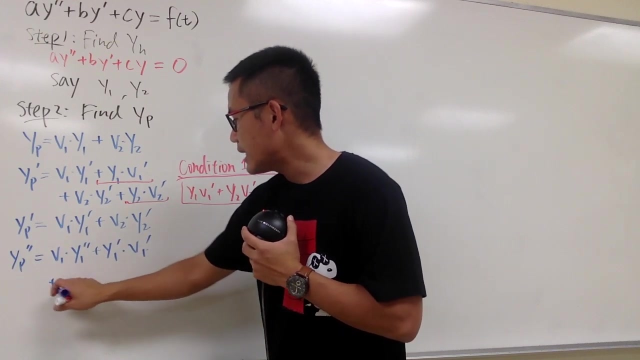 better. okay, so I'll keep the first function, phi1 times the derivative of the second, which is going to be Y1 double prime, plus the second function, Y1 prime times the derivative of the first, which is phi1 prime. and now move to here. let me add: 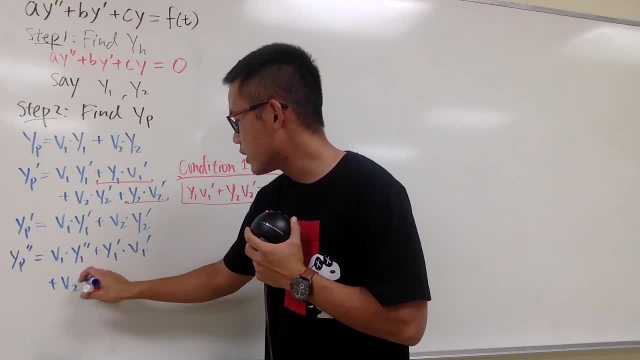 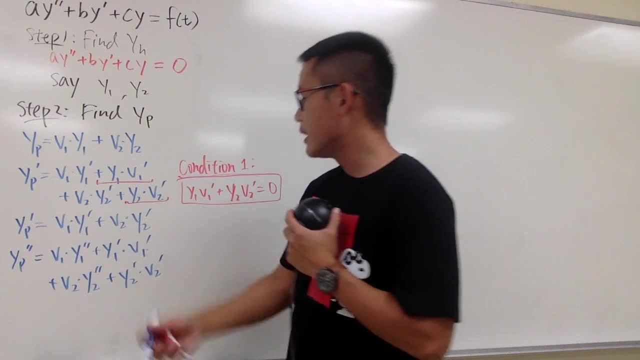 I'll keep the first function, which is phi2 differentiate, the second, so Y2 double prime, plus the second function, Y2 prime times the derivative first, which is phi2 prime. that's what we have for YP double prime and I'm not going to impose any. 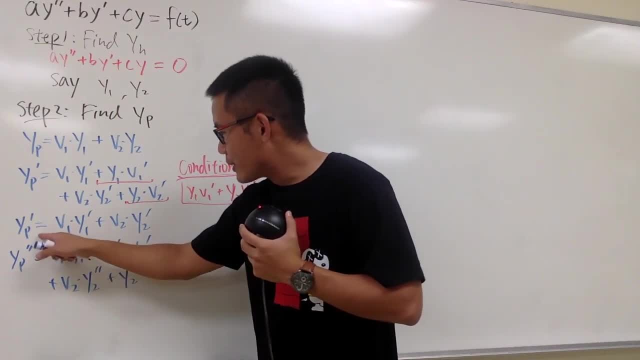 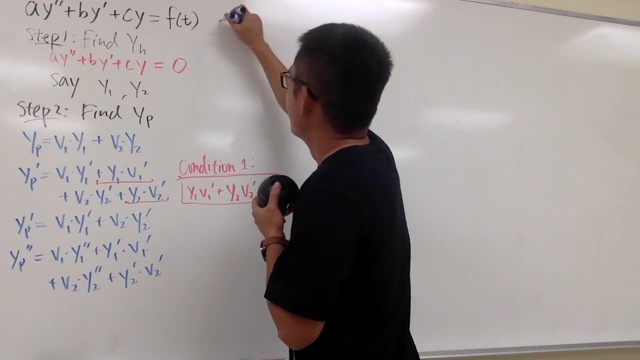 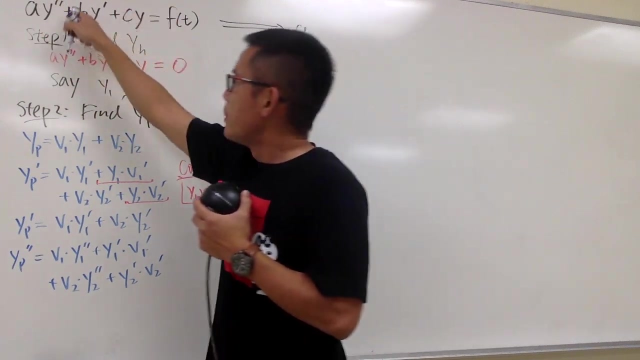 condition. I'm just going to look at this, look at that and look at this and plug in into the original and now let's see what do we get from here. so I have a in the front right here, times y double prime, which is this right and this? 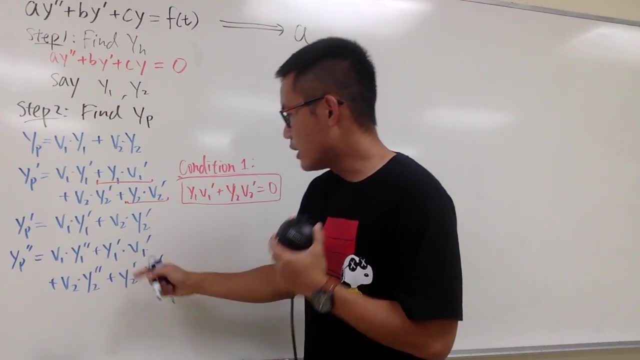 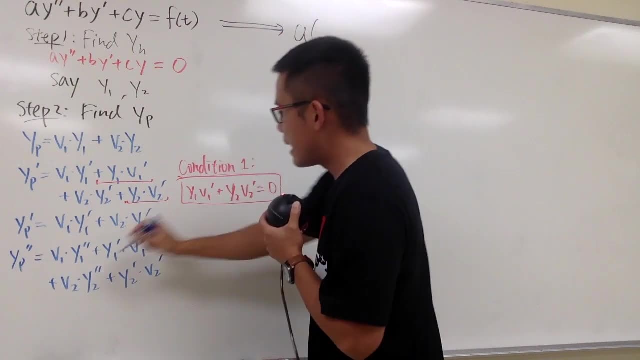 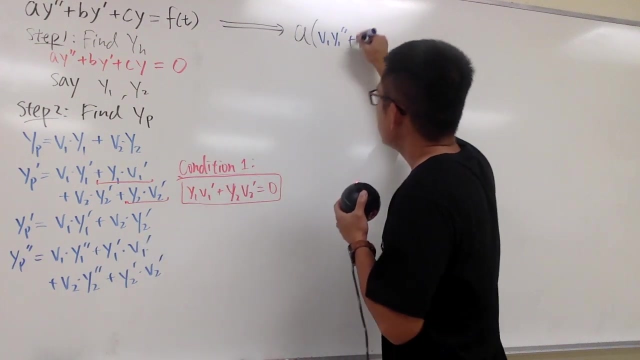 nothing I can do to compile a terms, then I will just put on all the fees first, if you guys don't mind. so let me write this down here. let me multiply by phi1, Y1, double prime, and then we add. as I said, I want to put on all the fees first, so let 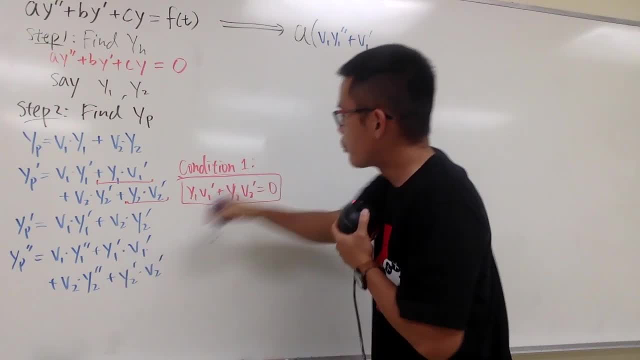 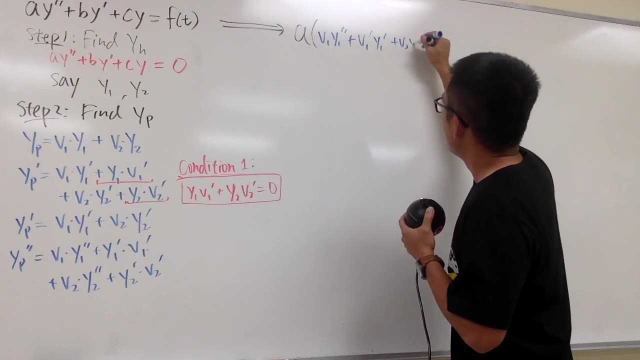 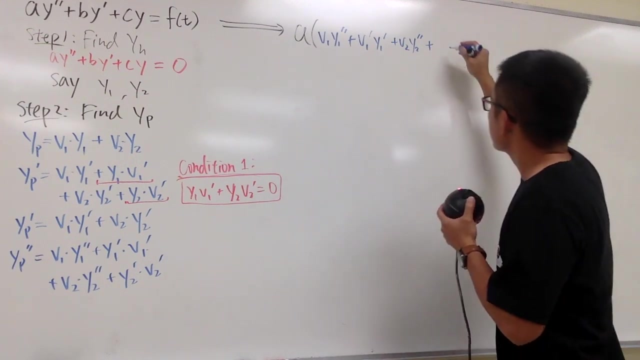 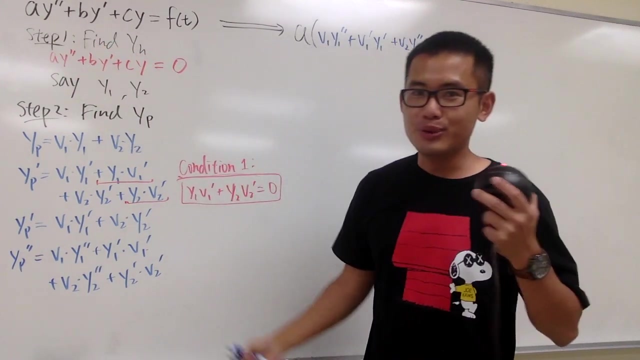 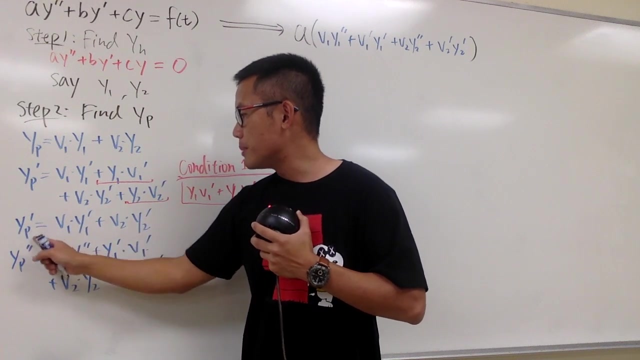 me put on phi1 prime, y1 prime, right, and then we have that which is v2, y2, double prime, and then we also add this with v2 prime, y2 prime, and this is that. what do we do? next, be y prime. and remember now, this is the y prime part, right because of the y P. 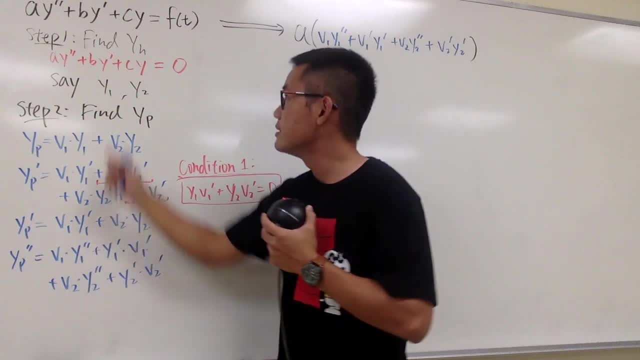 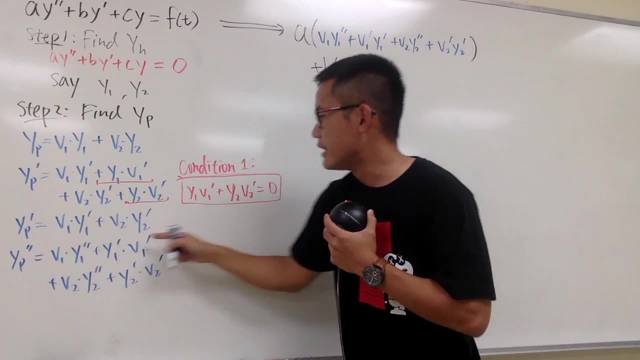 prime is just this. we have this condition, so we're plugging this into the y prime and then we just put it down below here, plus B times this, and that it's not bad at all, and if these are already in the front, so that's good. 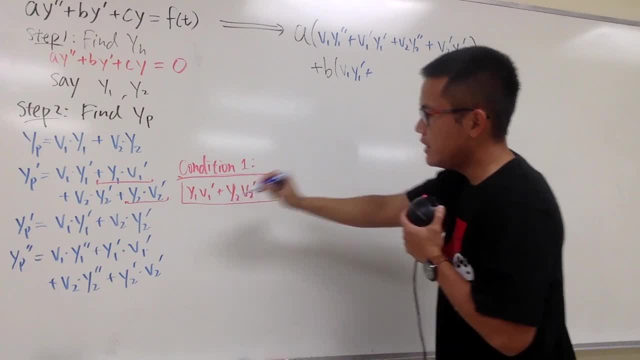 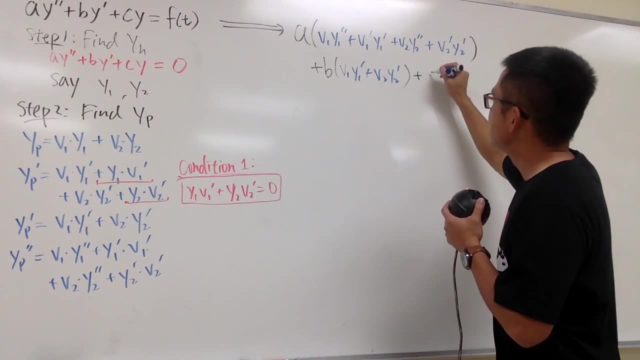 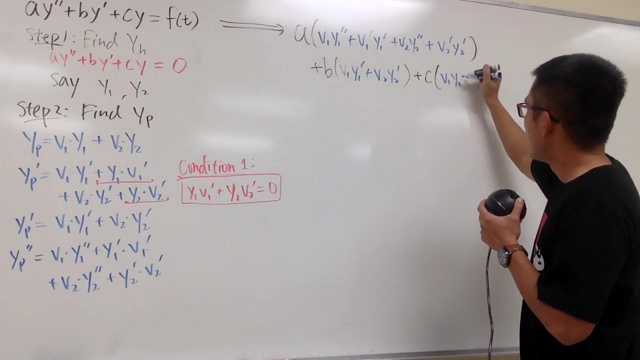 v1 y1 prime plus v2 y2 prime. okay, and now I will have to add C times Y and Y is just this. so that's over here, and then we have this condition. so we're opening the parentheses: v1 y1 plus v2 y2 and now altogether this is equal to: 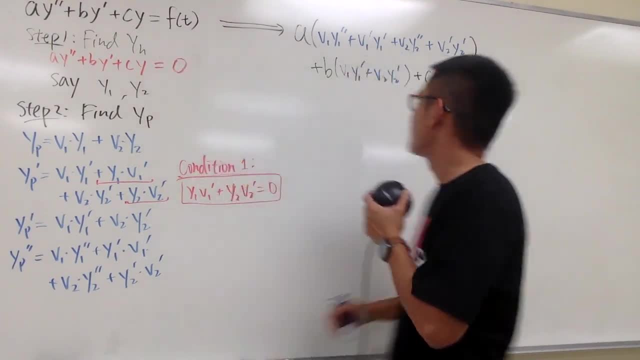 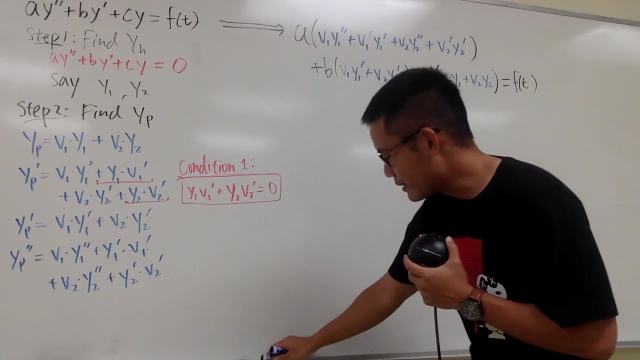 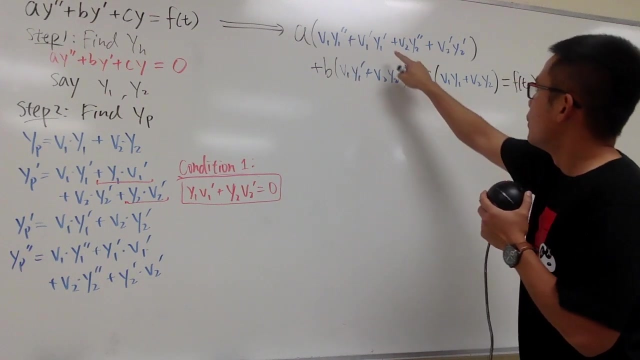 what f of T? because we're looking at the original, okay, and now what do we do next? let me talk about it, of course. right here's the deal. I see that I have the y1 double prime, y1 prime, okay, maybe, and then this is y1 prime and this is y1, but 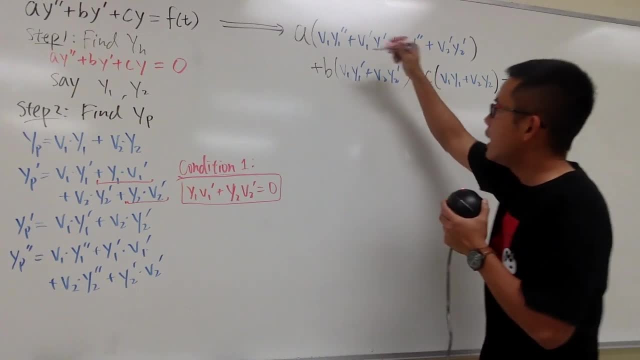 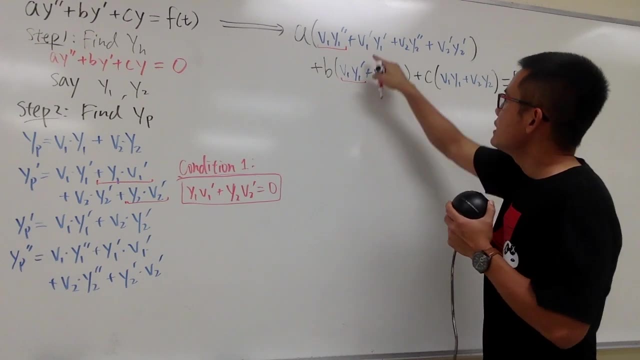 let me focus on this part, this part and this part. let me just underline this for you guys: this is v1 y1 double prime. this turn also has the v1 right. this one is v1 prime. I don't want to look at this. v1, v1 and this is also v1. 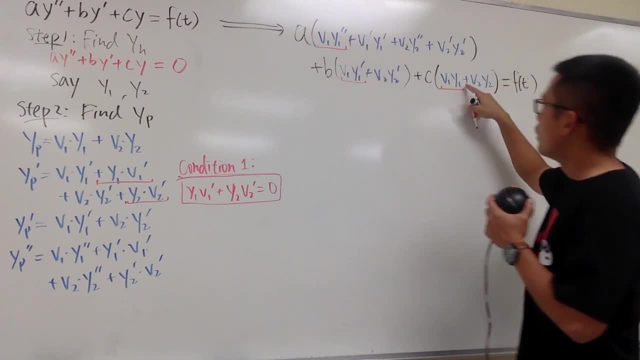 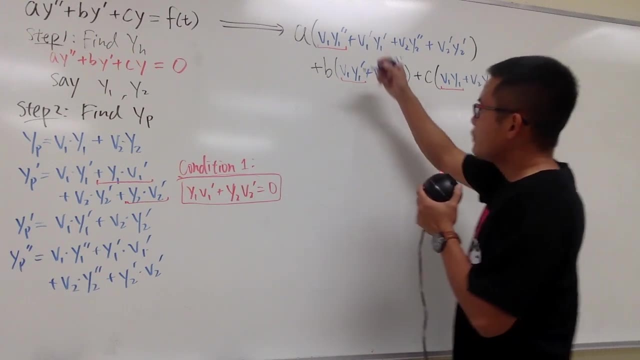 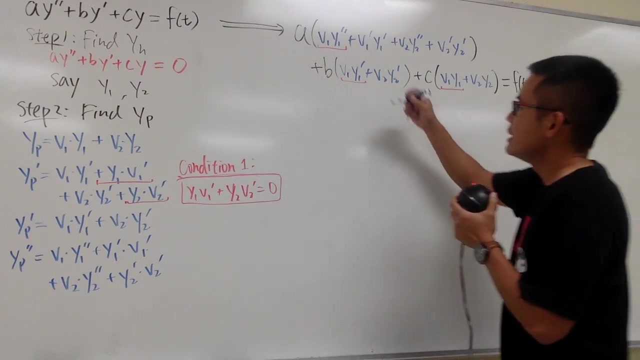 and then you see, this is y1, double prime, y1, prime y1. let's put them together and let's also factor out the v1. all right, and of course, don't forget, you have to distribute, distribute. we will have to do that, okay, and I will do this in black first, so I 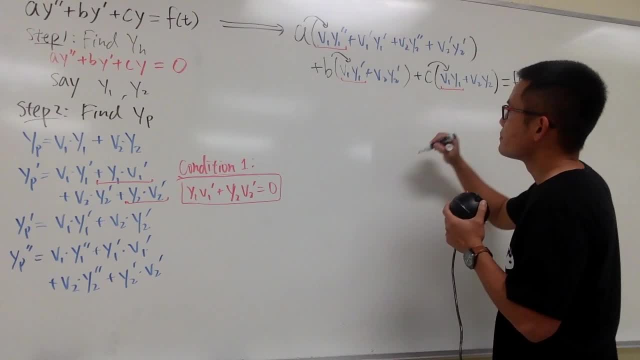 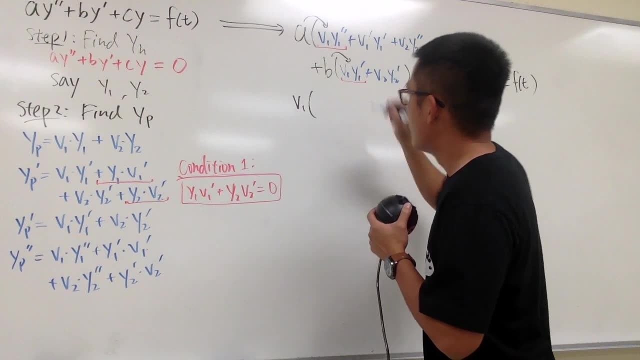 will say distribute, distribute and distribute. I am going to factor out the v1 first, so let's put this down in the front. we have the v1 right here. I'll open the parentheses and let's see this v1 is in the front already. I would like 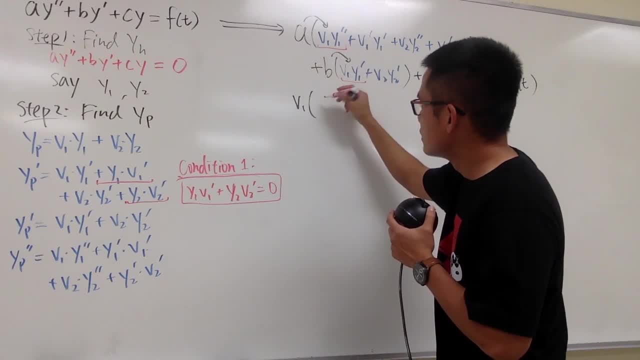 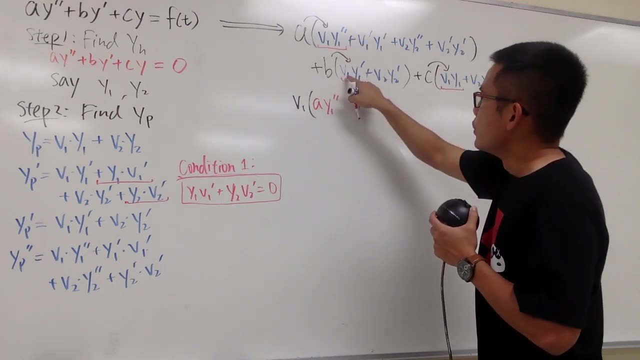 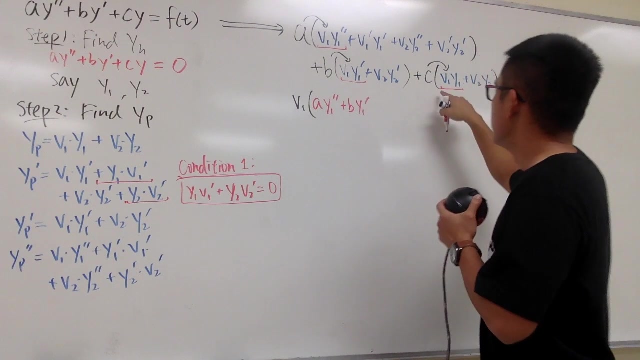 to put down a y1 double prime right here for you guys. so a y1 double prime right here and next. you see, we took out the v1 already. this is plus b times v1 prime. so let's put down plus b y1 prime likewise for this term. we took out the v1 already. 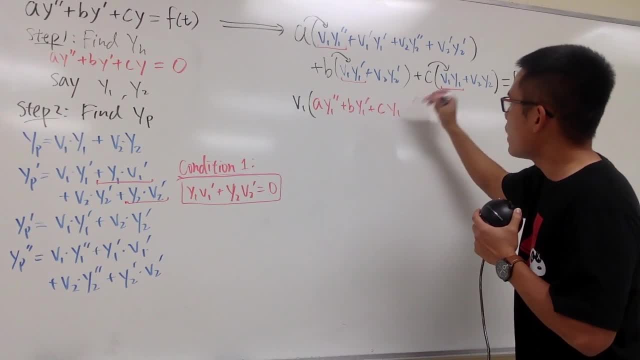 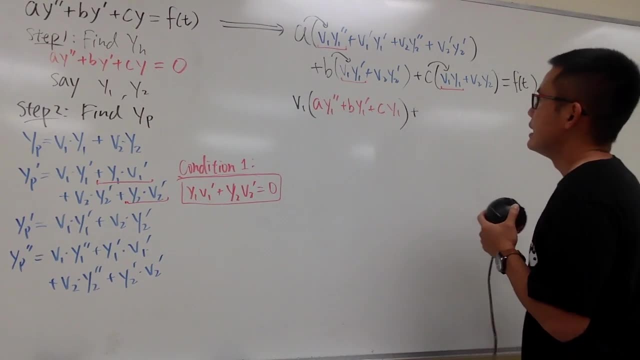 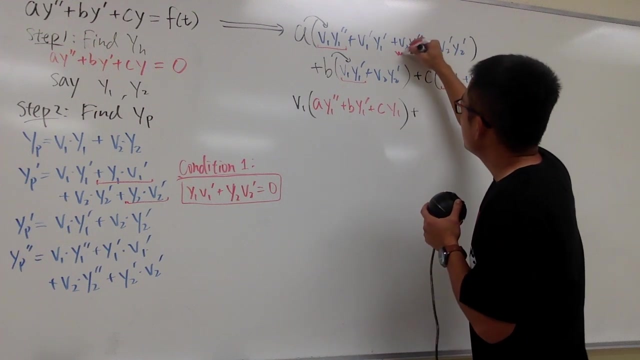 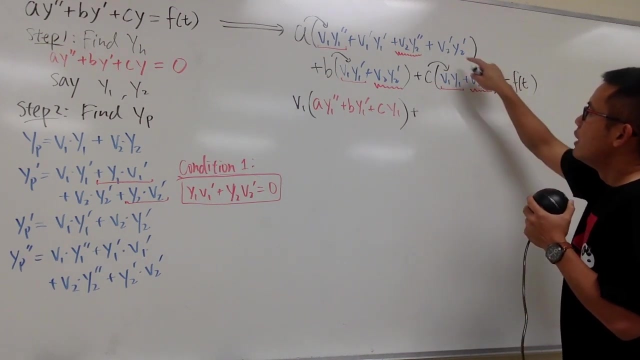 so we have this and that plus c y1, that's it right. and now, next, we will just say: let's add, let's do the same thing here. let's look for the y2s. I see that I have this v2 y2 double prime, and then v2 y2, prime, and then this is v2 y2. I don't want this. 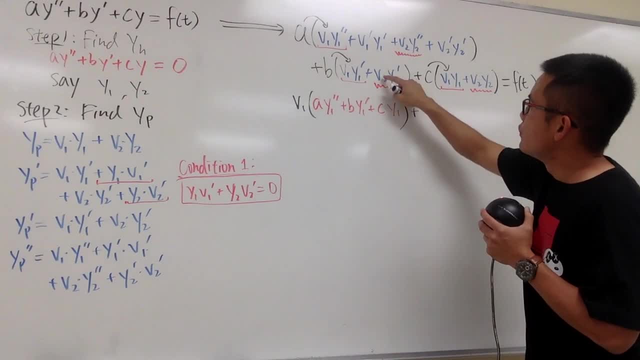 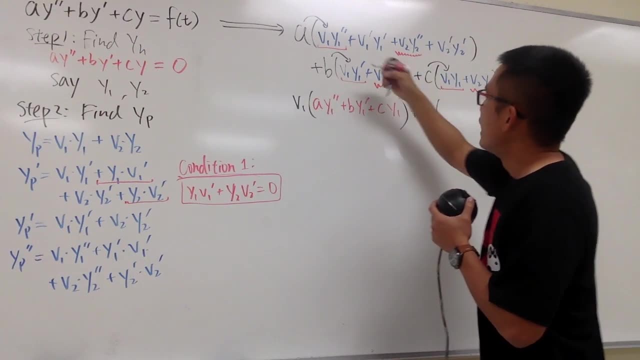 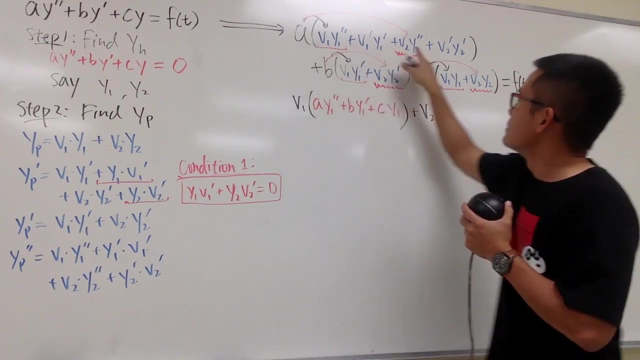 because this right here has v2 prime. this is v2, v2, v2, so I can factor out the v2. okay, so let me do that, let's factor the v2 first and then I will do this times that, this times that, this times that, so a times y2 prime that will go here, because the v2 is out already. so we will have. 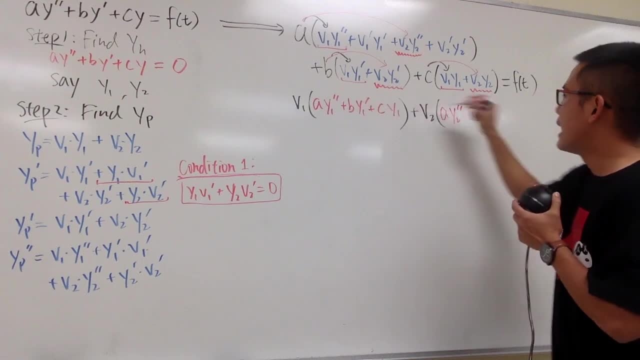 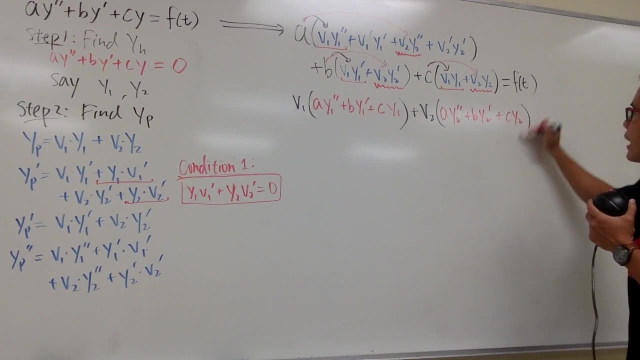 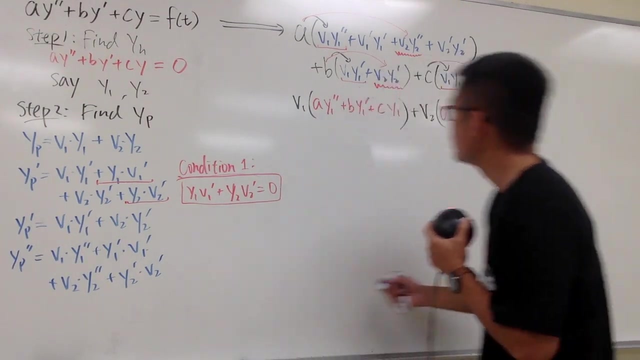 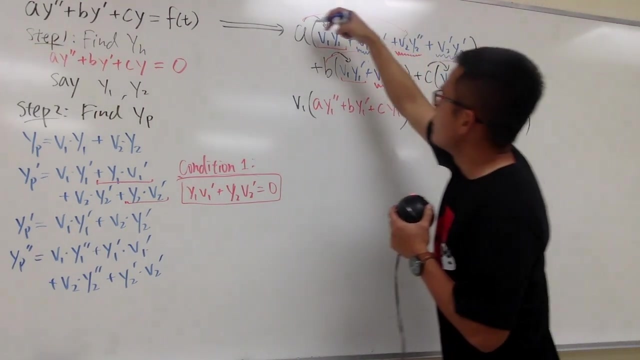 a- y2, double prime, and then this times, that is plus b- y2, prime, and likewise this, and that it's just plus c- y2. okay, all the v2s are out already. lastly, what do we have? well, I'll put this down in blue, as you can see. this is the remaining part, right in blue. this and that, and don't forget you. 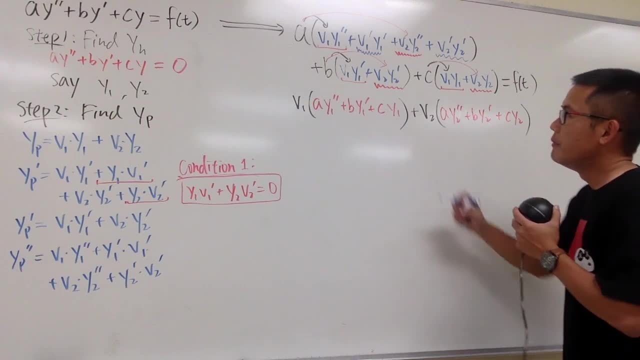 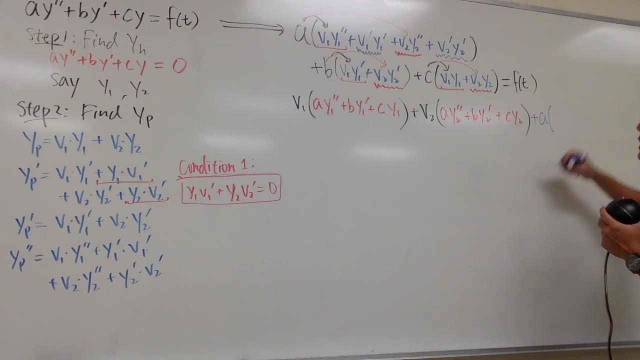 have the a in the front. I'm not going to distribute it, let me just put it down as a on the outside. so let me just put this down: plus a on the outside, parenthesis: phi 1 prime, y1 prime. so that's right here and then. 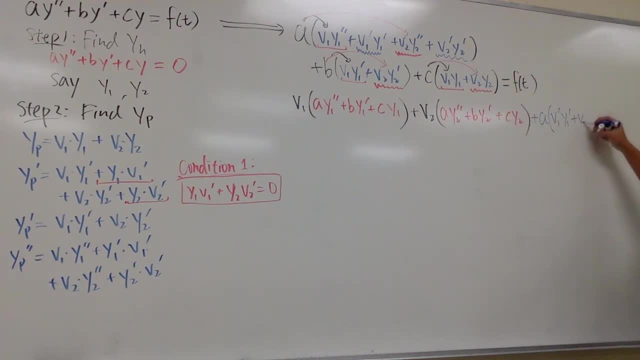 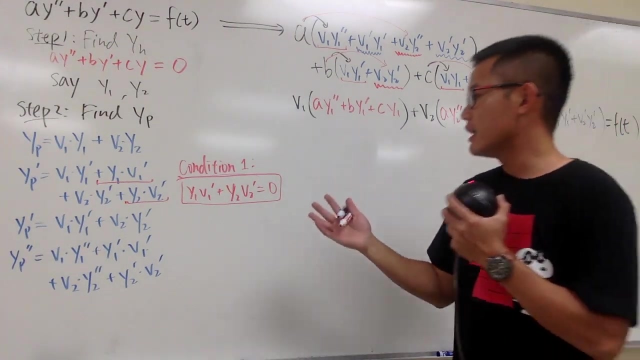 this is phi 2 prime, y2 prime, and they are both inside right. that's what we have and keep in mind. all this is still equal to f of t. okay, so it's not bad, because a lot of things have actually, you know, good patterns. 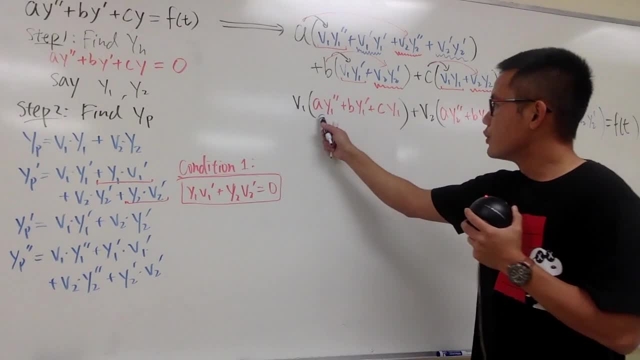 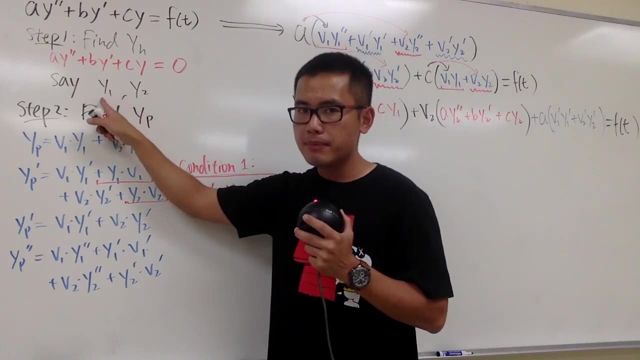 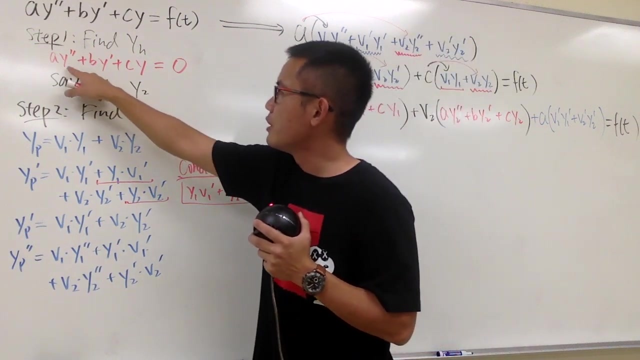 and all the good things. anyway, do we recognize what this is going to be? well, what does y1 represent? remember y1, it's a solution to the homogeneous equation, right? that means, if you plug in y1 to here, here and here a. 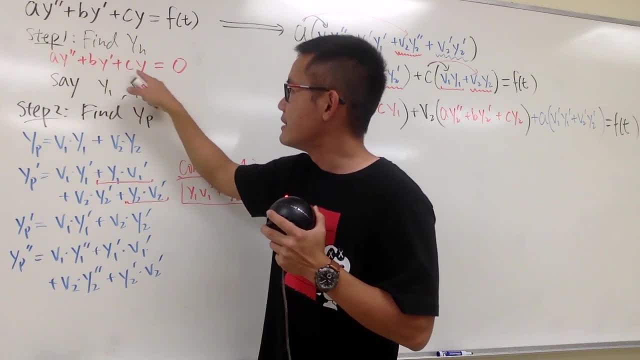 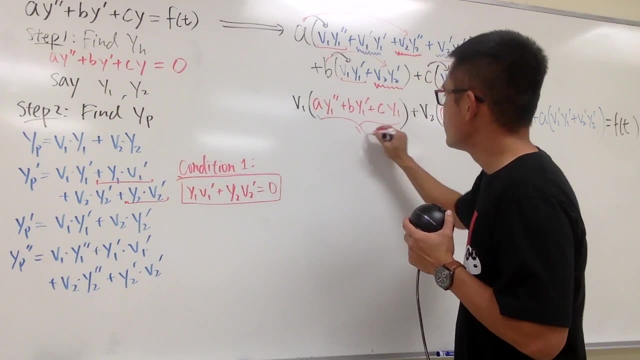 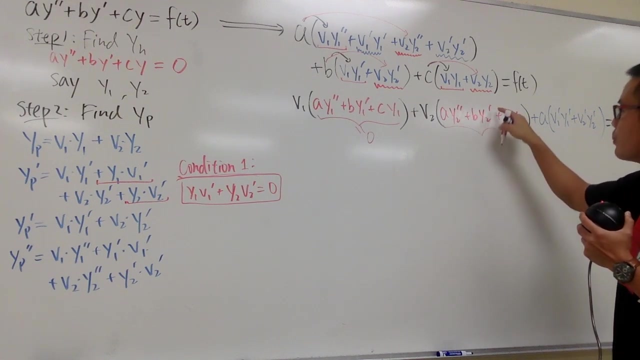 y1 double prime plus b, y1 prime plus c. y1 should be equal to zero, isn't it? so all this part is actually just equal to zero. and likewise, if you look at this right here, a, b, c and we have the y2 prime, y2 prime. 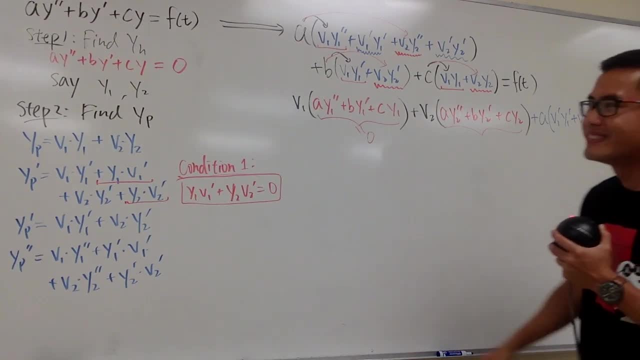 so this is y2 double prime, y2 prime and this is y2 that situation. this will also give you zero, isn't it? and all in all you just have. this is equal to that right. and now let me just write this down right here for you guys. we have: 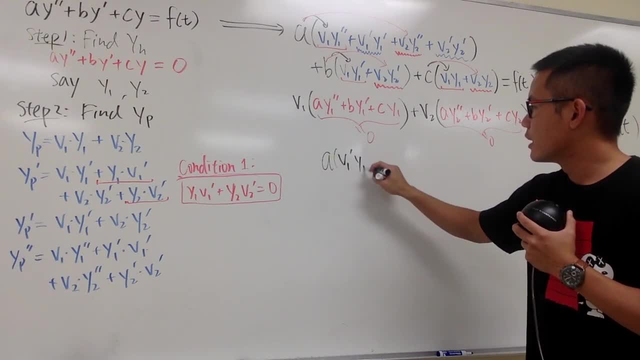 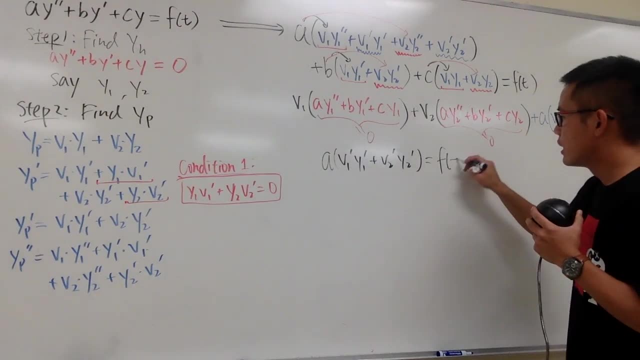 phi1 prime, y1 prime, plus phi2 prime, y2 prime, and this is equal to f of t, and of course we can divide by a on both sides. so in other words, we will have this: equals to f of t over a, in fact. 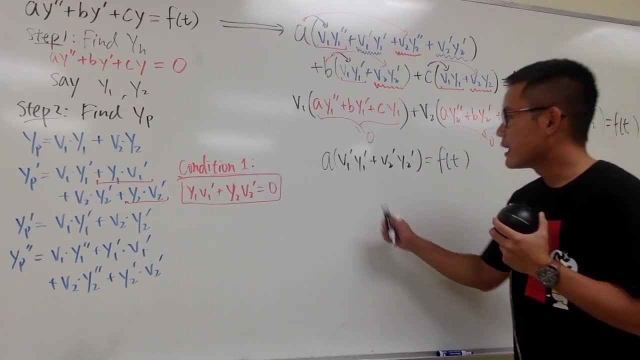 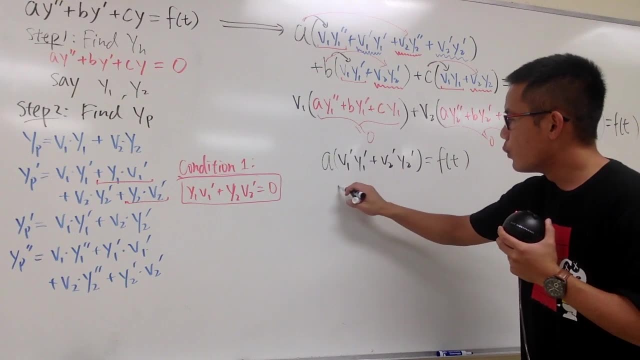 that will be the second condition that we have to impose. but let me do two things right here. first of all, let me switch the order so I can match that. okay, let me put down y1 prime first and then the phi1 prime. 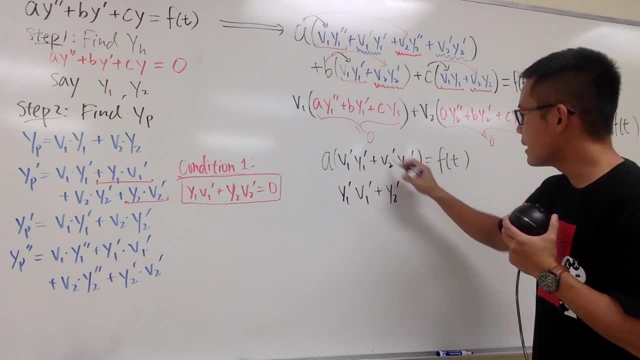 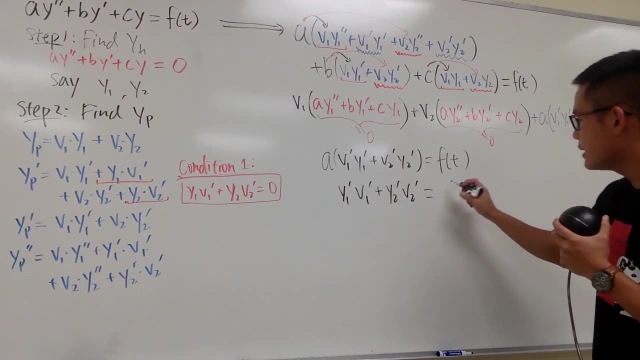 and then we add it with: let's put down the y2 prime and then the phi2 prime, and this is equal to, as I said it we divide by a on both sides. so on the right hand side we'll just have f of t. 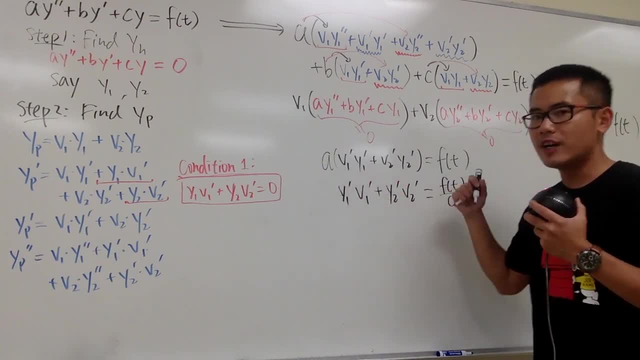 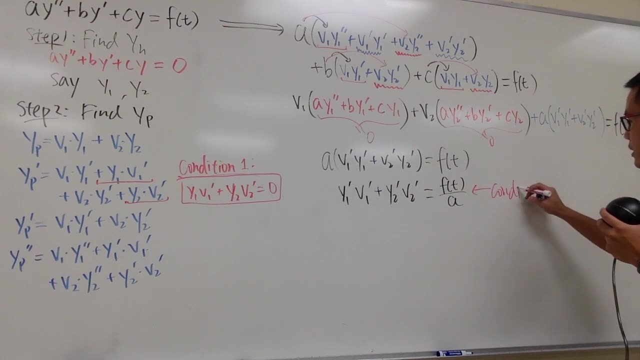 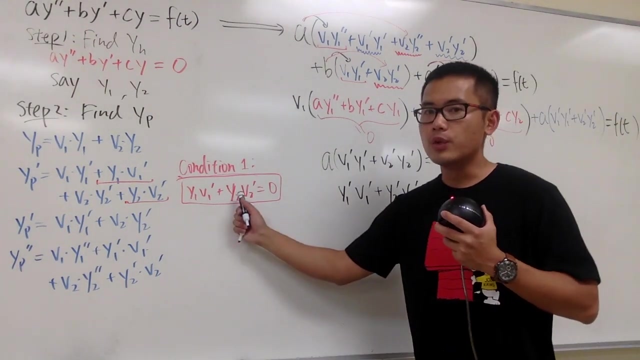 over a right, so we switch the order and also divide by a on both sides, and this right here is exactly condition 2. let me just indicate that condition number 2, okay. so, all in all, what we want to do is we have to solve this system. 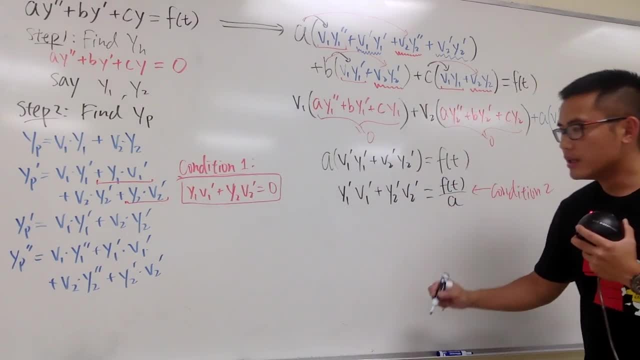 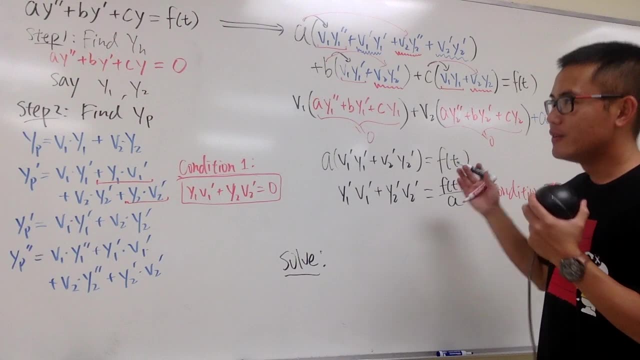 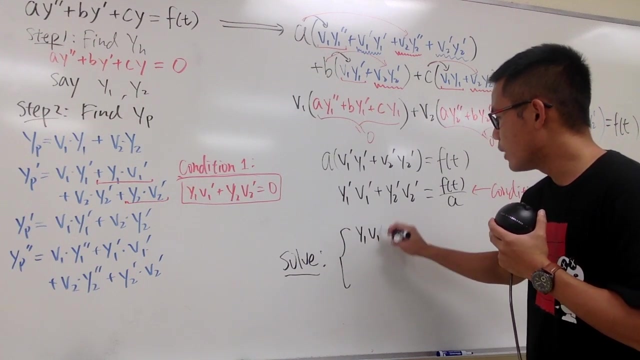 equation: this condition and that condition. so let me just put this down right here. whenever you're trying to do the variation of parameter method, what you have to remember is first condition, which is y1 b1 prime plus y2 b2 prime equals to 0. 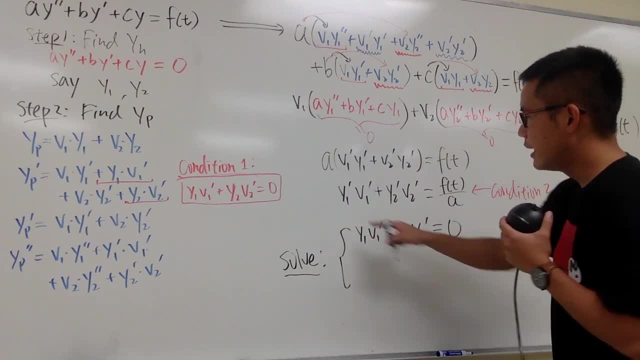 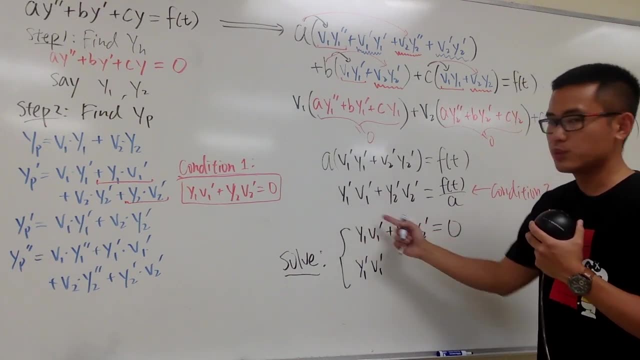 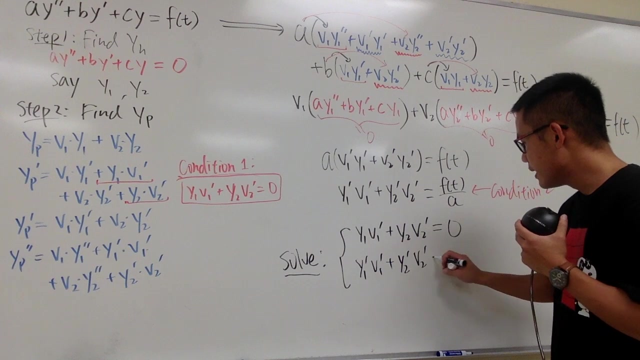 and the second condition is this: and you see, we have the y1 prime and then the phi1 prime, and you see, this is the reason why I switched the order, so I can light them out nicely right, plus y2 prime, and this is phi2 prime. 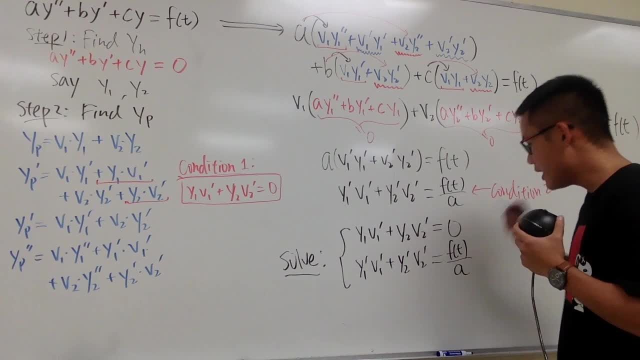 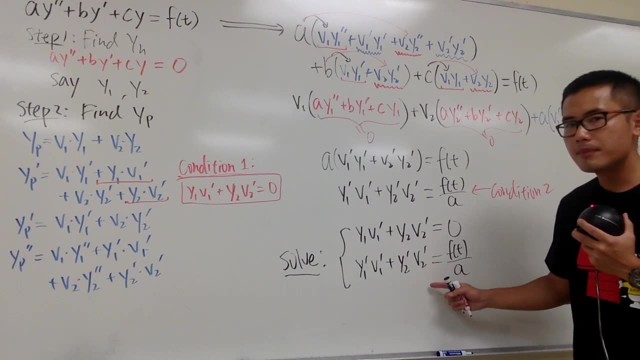 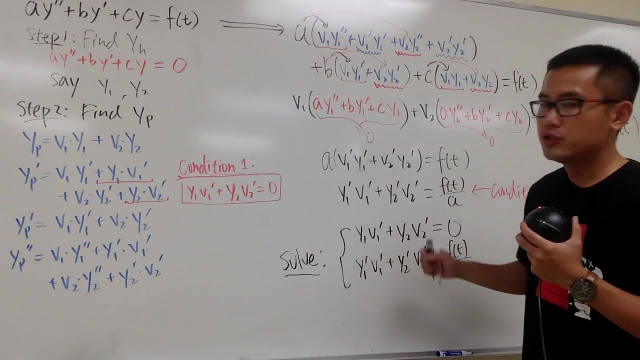 equals to f of t over a. from here you should be able to solve for phi1 prime and also phi2 prime, because this is just a system equation and y1, y2, y1 prime, y2 prime should be easy to get. 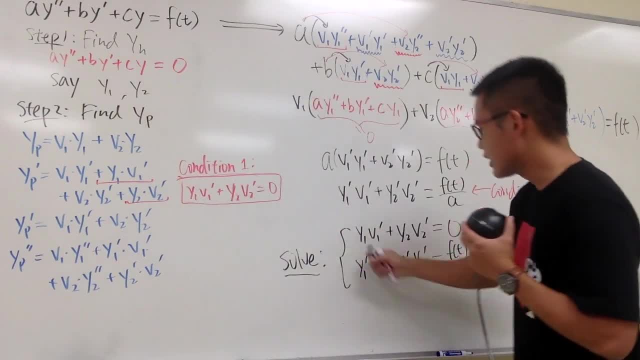 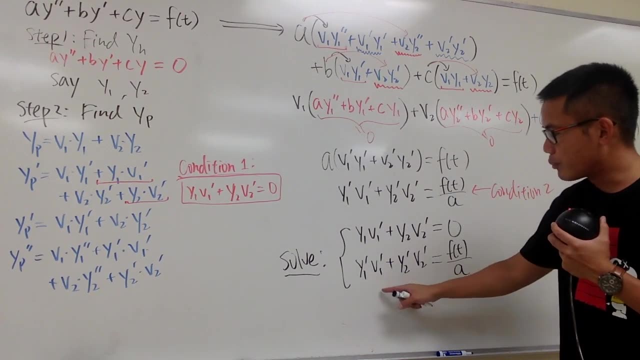 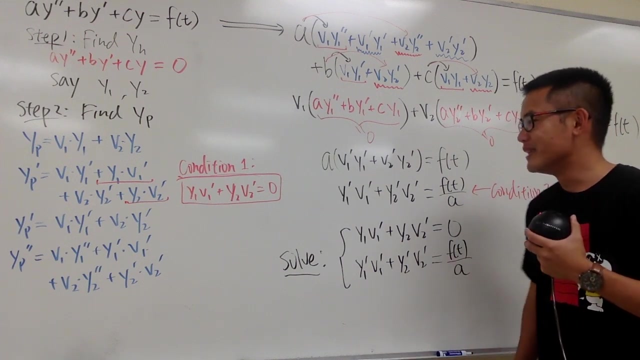 because it was easy to solve this right. so you just have to put the functions here here and the derivatives here and here, and once you are able to solve for phi1 prime and phi2 prime, you can integrate to get phi1 and phi2, and things like that.